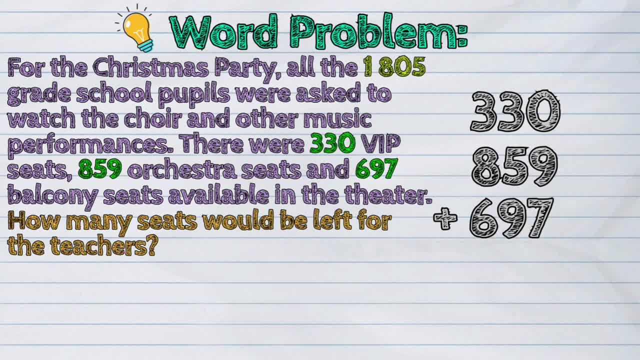 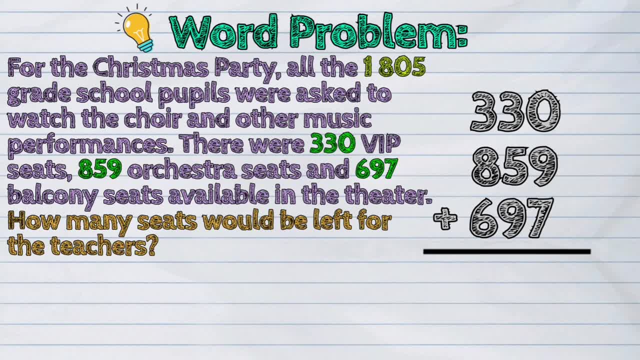 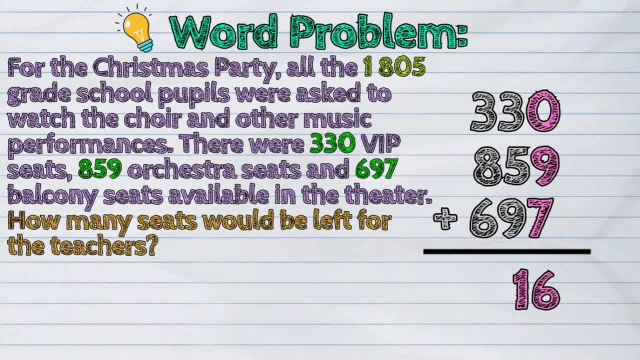 place Sixteen. We will regroup this number by putting six ones as the answer and carrying one ten in the tenths place. Now the sum in the tenths place is Eighteen. We will do the same process of regrouping. 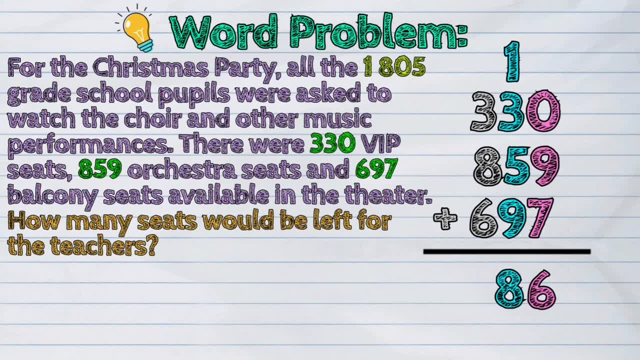 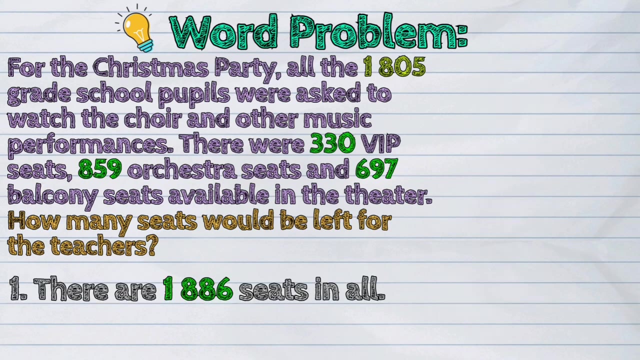 Put digit eight in the tenths place and carry one in the hundredths place, And the last column is the hundredths place. The sum of the numbers is Eighteen. So there are 1,886 seats in all. Let's proceed now. 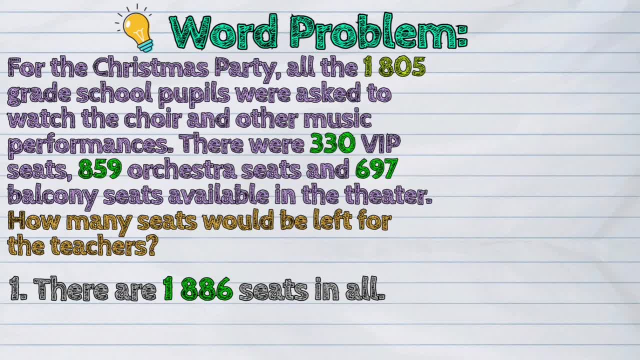 Let's proceed now to step two. To find out how many seats would be left for the teachers, we have to subtract the number of grade school pupils from the total number of seats we solved in step one, So it's 1,886 seats minus. 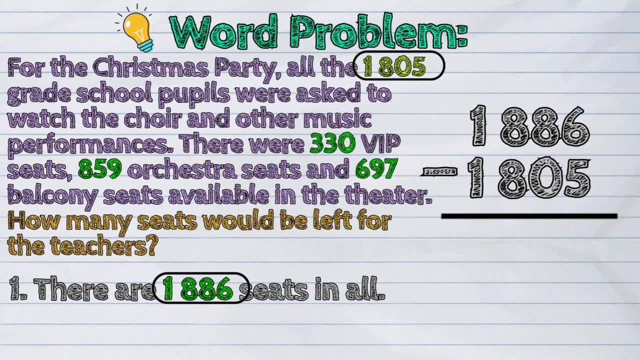 1,850.. to find out how many seats were left, The difference in the ones place is One, In the tenth place is Eight, In the hundredths place is Zero And in the thousandths place is zero also. 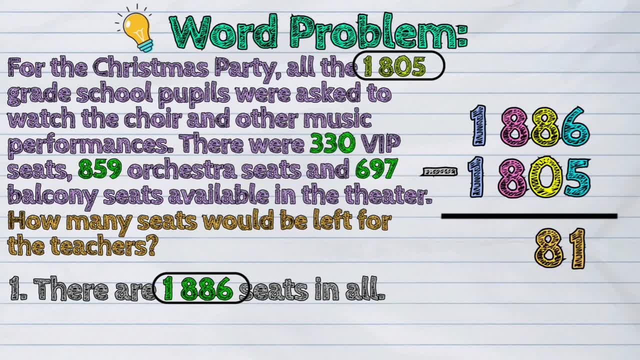 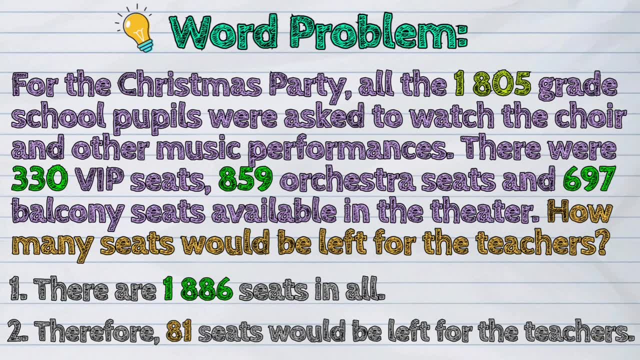 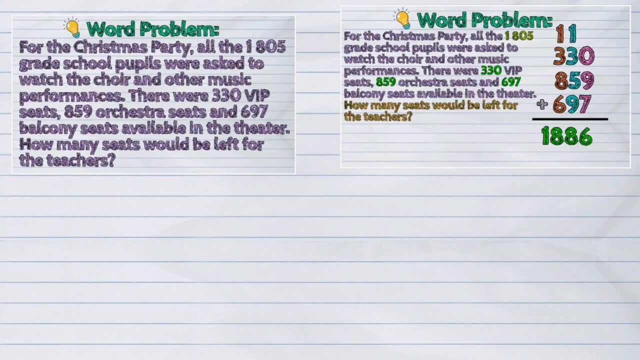 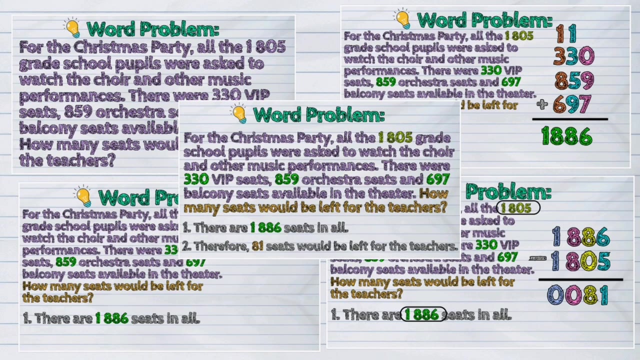 So the total number is Eighty-one. Therefore, 81 seats would be left for the teachers, And that was how we solve a two-step word problem involving addition and subtraction. Take note that there are really word problems that require you to solve two different equations before coming to the answer.